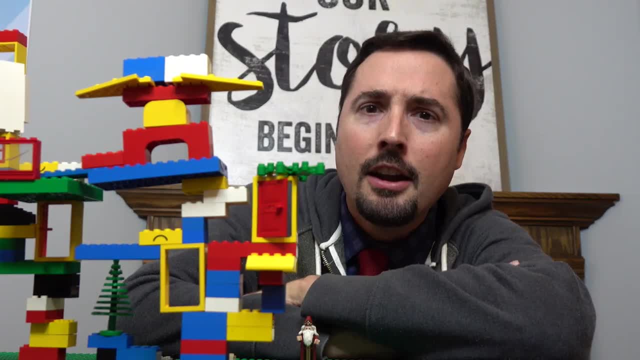 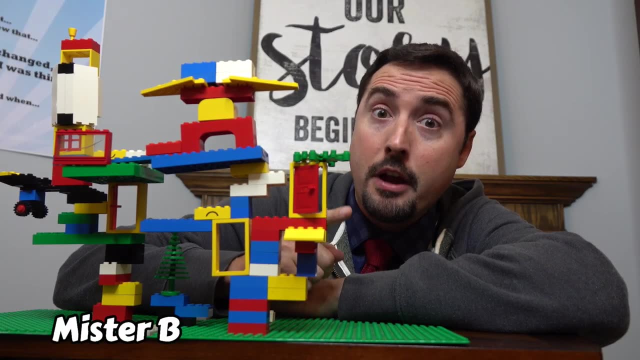 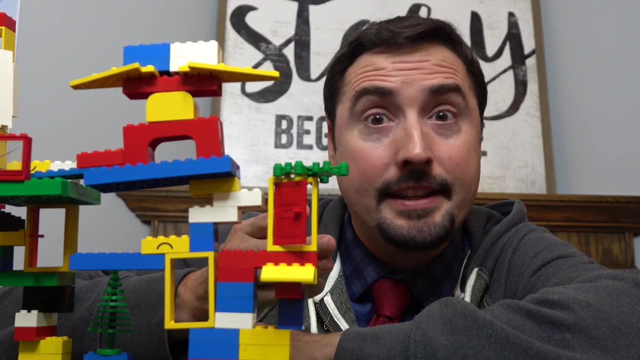 Building things are kind of fun. Are you the kind that likes to make up your own thing or follow the instructions? But the one thing about your ideas is that if you're not careful your structure can be unstable. No, It happens to the best. You see, I got this Dumbledore and I figured he needs a. 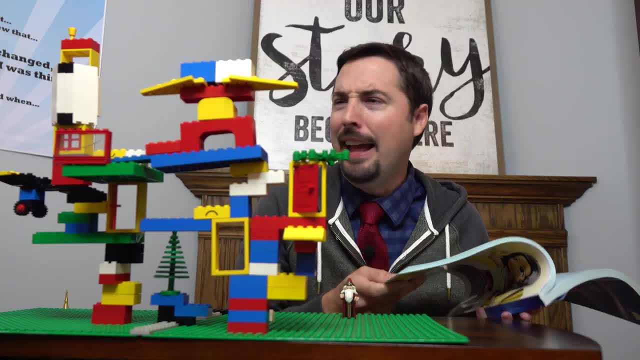 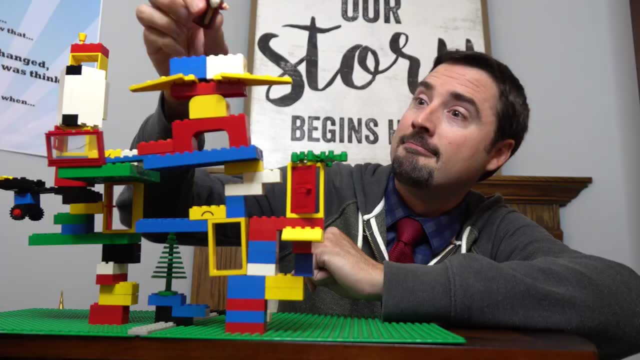 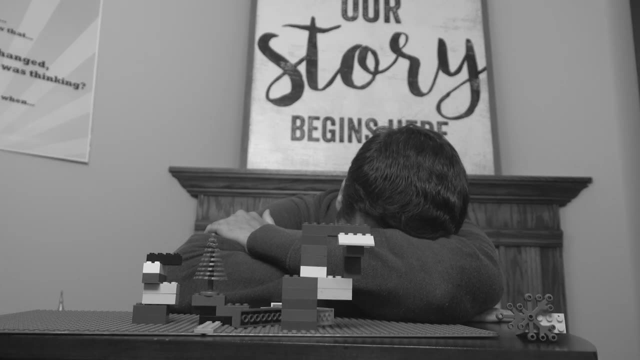 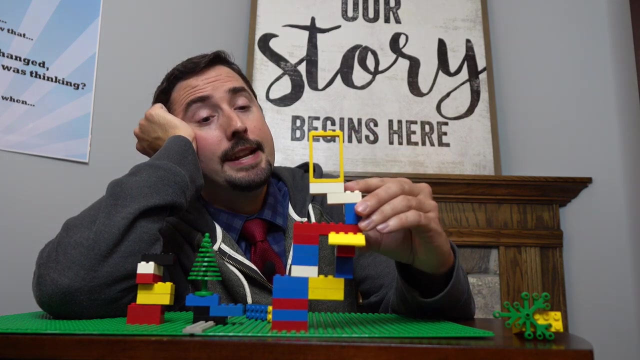 Hogwarts castle. But the instructions for this thing are insane. I think I can just look at the picture and figure it out And when I finish, Dumbledore is going to look great in his tower. You know, stories are like building blocks. You might have the right elements of fiction. 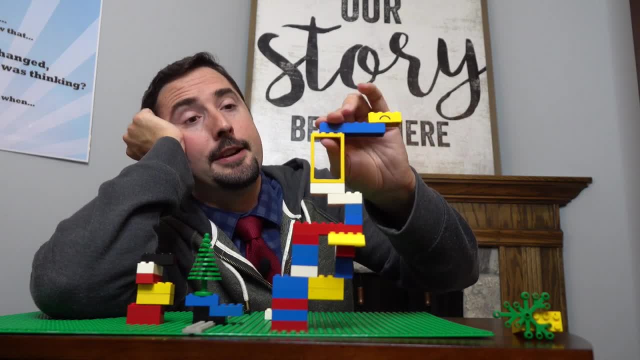 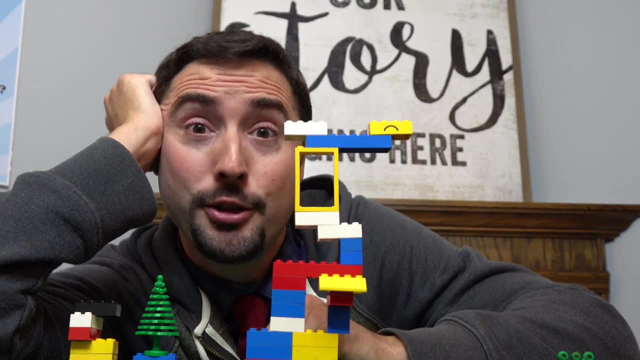 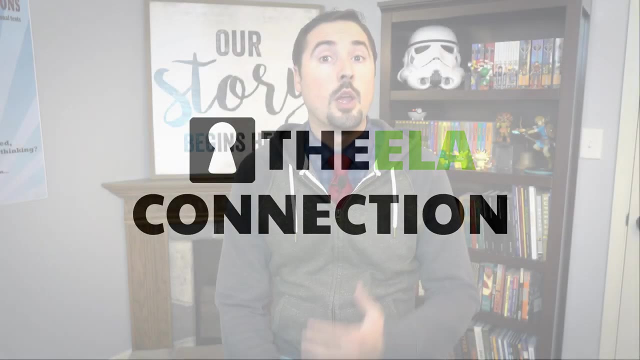 but if you don't have good structure, it's not going to work out so well. I guess I'll start over and use the instructions this time, but let me cut Connect this to how good stories need good structure. We all know that every good story has to have plot, But what does that mean? Well, 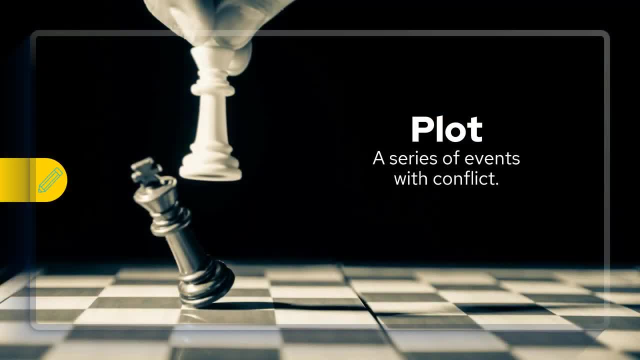 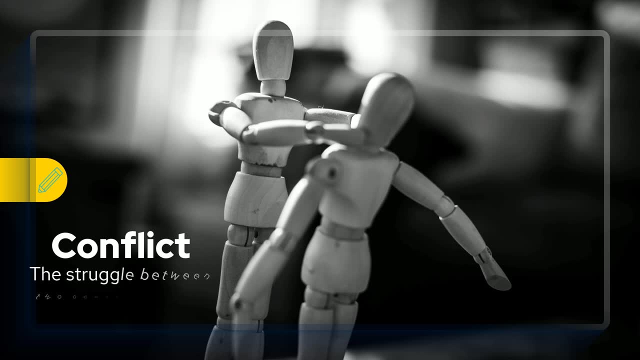 let's talk about plot structure. Plot is a series of events with conflict, And every good story has a problem that must be solved. We call that conflict. Without it you get boring stories, You know, kind of like the ones you read in English. 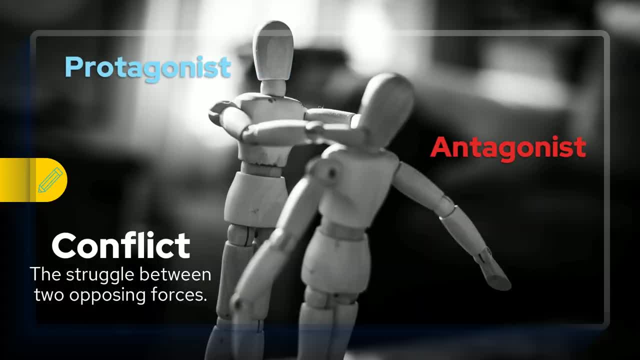 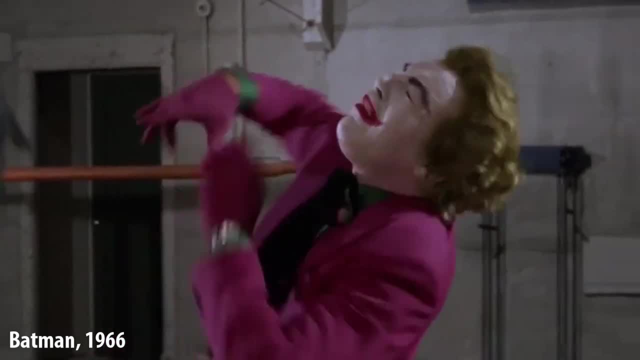 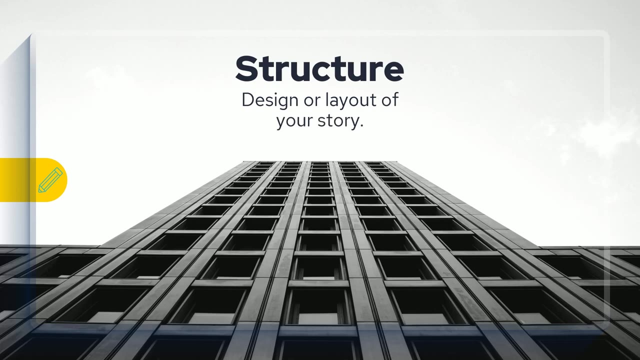 But conflict is often between a protagonist and an antagonist. That'd be like Batman finally stopping the Joker from one of his dastardly plans. But stories need good structure. That's the design or layout of your story. So what kind of structure do all stories have? Well, they all have a beginning, a middle. 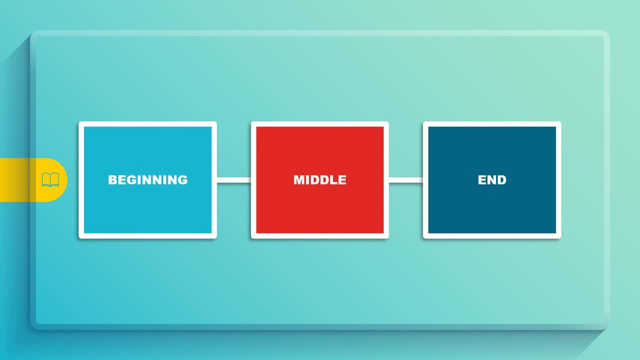 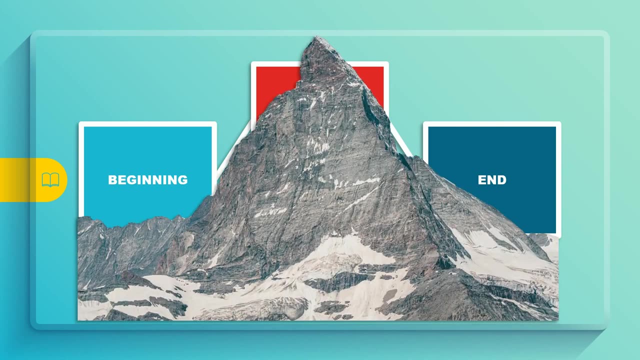 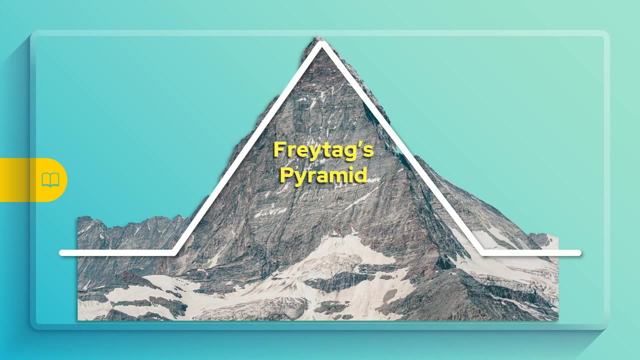 and an end. But this structure does not indicate that there's any conflict. It's just three events. So let's visually represent conflict by bumping up the middle, And well, we start getting what appears to be a mountain shape. Let's trace the outline of this mountain and what do we get? Freytag's Pyramid. Wait a second. 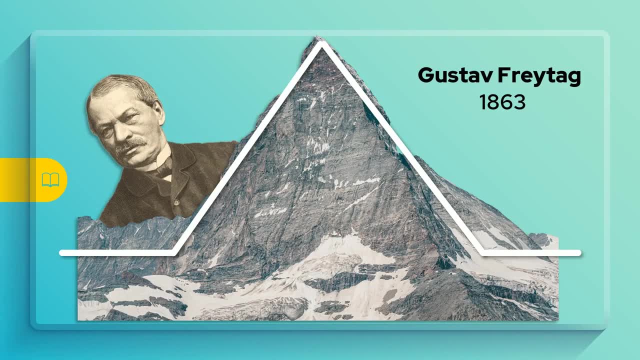 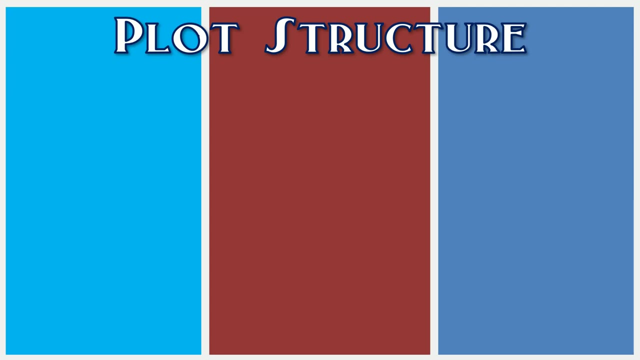 who in the world is Freytag? Glad you asked. Gustav. Freytag is a German author, and in 1863, he created what we consider a universal structure for stories, And he's been torturing students with it ever since. He believed good stories have two major parts: the beginning and the end. 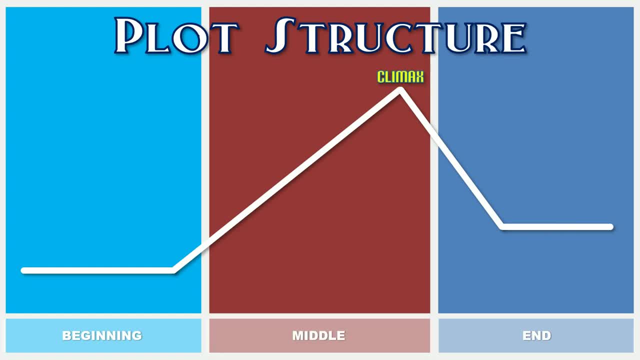 but with a climax that takes place between those two. That leaves us with five other parts of his structure. We've got exposition, inciting incident, rising action, falling action, and the resolution, or denouement, if you're French. Let's take a look at each of these in detail. Exposition: 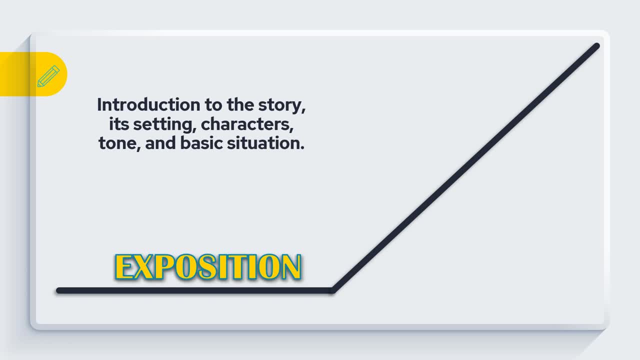 is the structure of a mountain. It's a structure of a mountain. It's a structure of a mountain. It's the beginning of your story. It's where basic story elements are introduced. We see where it's taking place, we meet our main characters and usually there's a basic situation, But one. 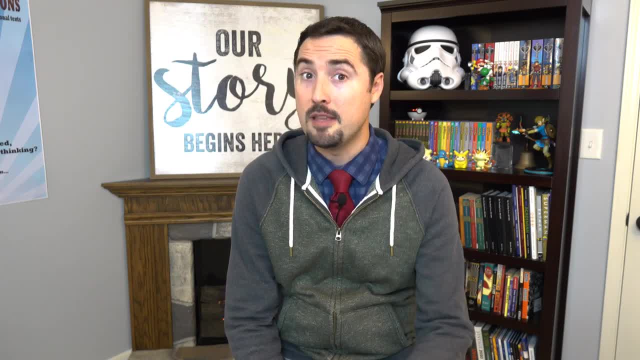 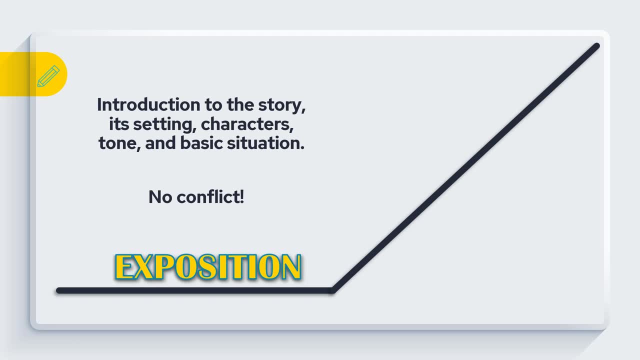 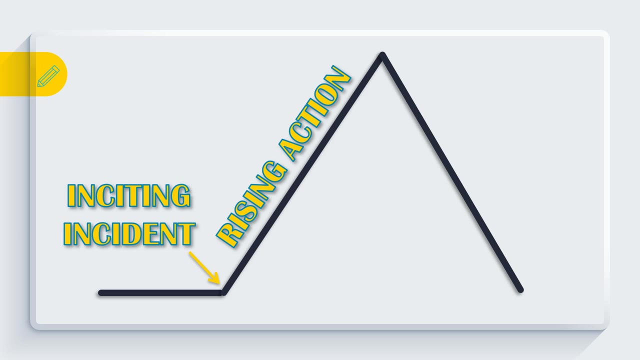 thing that you're not going to find in the exposition is the main conflict. That's why, you see, the line is flat. There is no conflict. Exposition simply sets the scene and story, But remember, we've got to introduce conflict. So shortly after that exposition we hit that mountain. 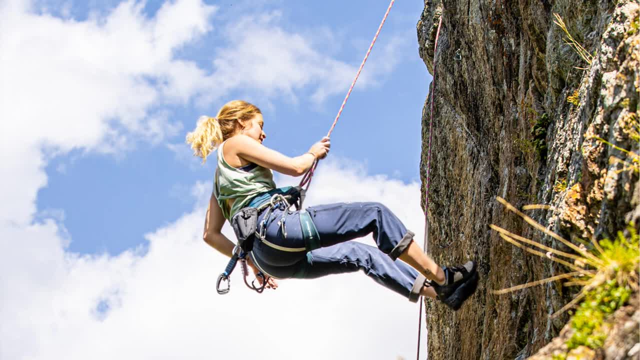 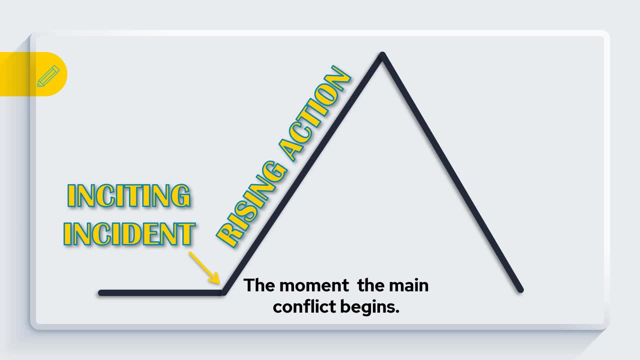 And just like climbing a mountain in real life, climbing the story mountain means conflict. The inciting incident is that very moment where a force requires the protagonist to take action, which leads us right into rising action. Each step in your story should build in action. 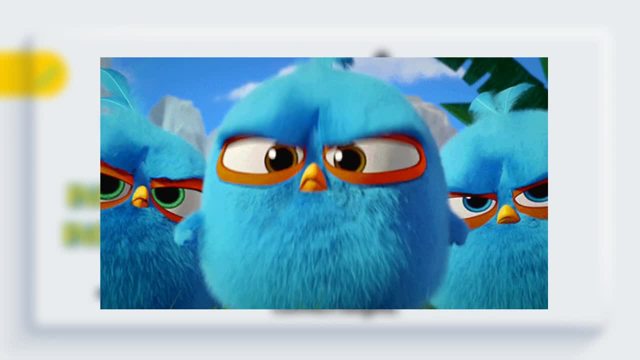 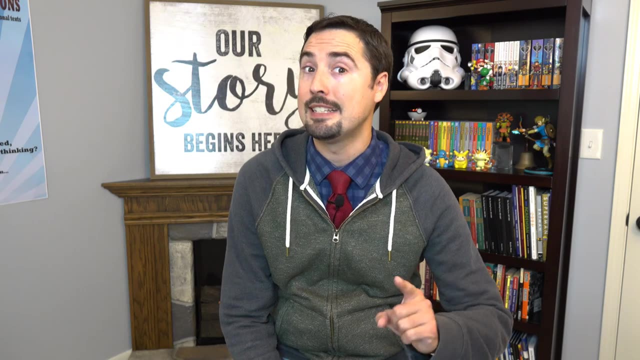 They might meet new characters along the way. They might have a lot of conflict to face, But as the story progresses we should see conflict escalate. Climbing a mountain is a lot of work, so our characters should go through a lot of conflict in the story. Finally, we are at the 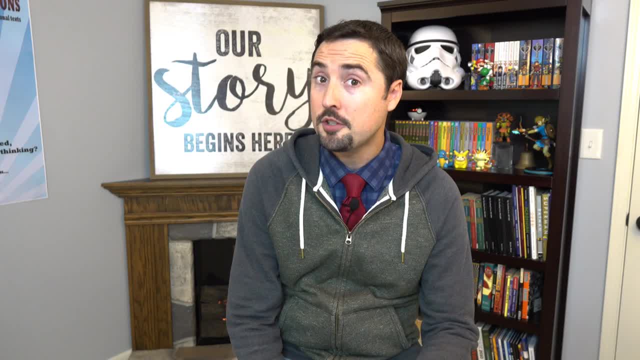 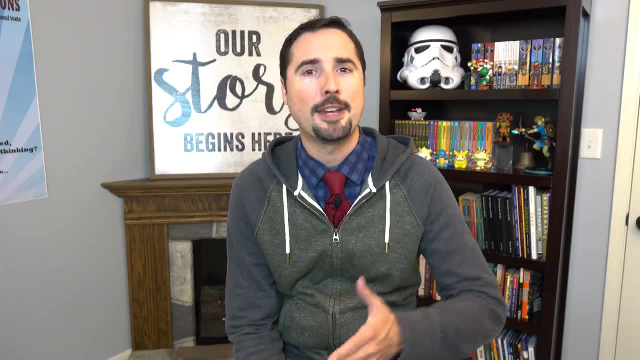 top of the mountain and it's called the climax. But this is not a place to rest. Oh no siree. This is when the main conflict is the strongest. Let's visualize this with some characters. Our hero has made it to the climax of the story. He's gone through a lot to get here. 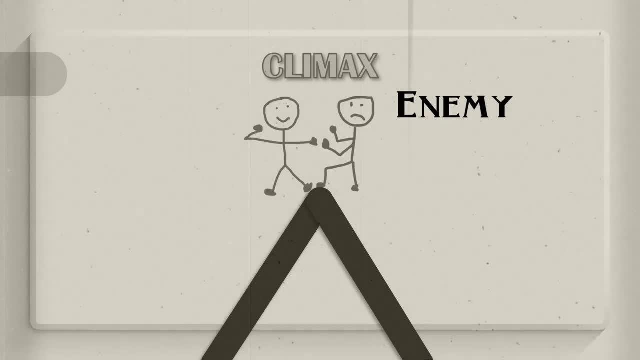 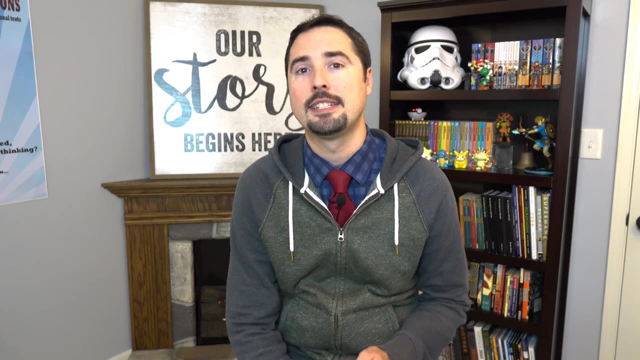 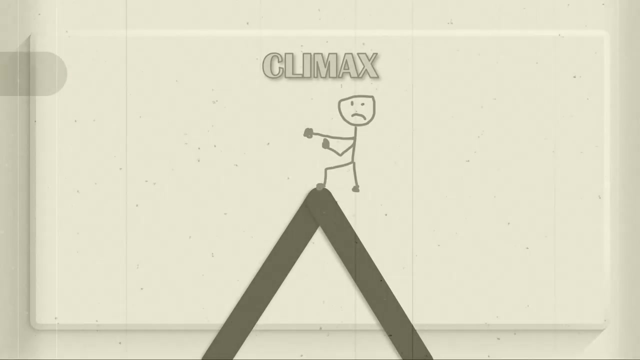 but now he must face his enemy, the antagonist. During the climax, the conflict appears to be its strongest, and that's when all hope appears to be lost. Oh Ouch, Oh no, Our protagonist has just fallen. Is it over?